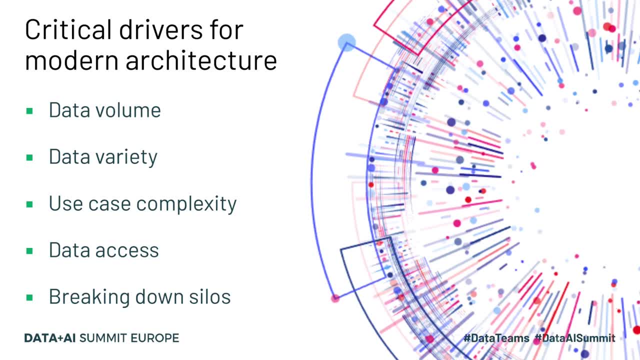 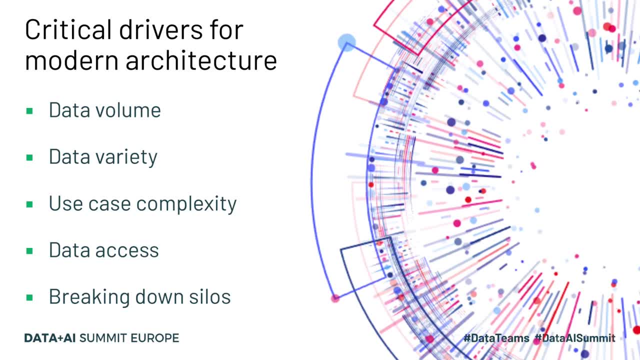 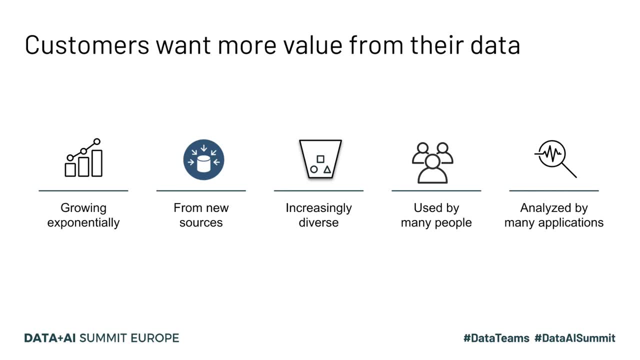 Data needs to be available. Data needs to be available in one common location. Customers want to have more data from their value. As I mentioned, data is growing exponentially and it comes from many new sources and it is increasingly diverse and used by many people, with many different people of many different roles. 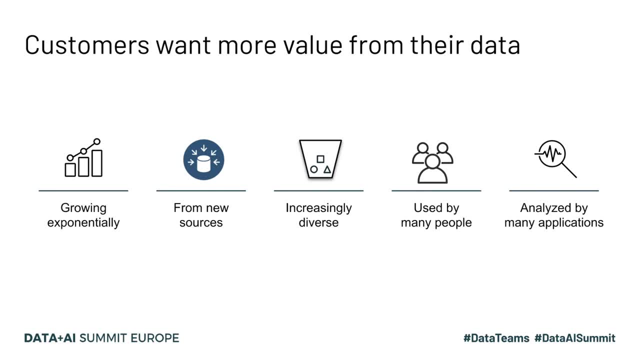 You have data engineers, you have data scientists, you have analysts and you have users who are only familiar with user interface. You are also familiar with states driven data analysis, And data is analyzed by many application. You can, for example, have different BI tools connected to the same data set. 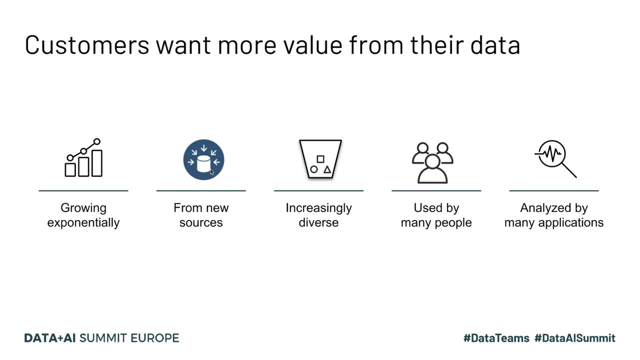 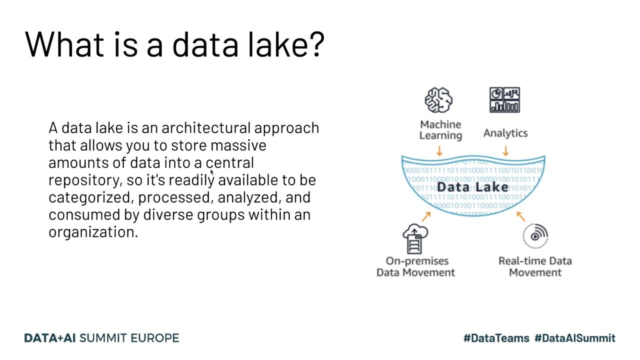 Different users may have their own tools that they have. data analysis. What is a data lake? A data lake is an architectural approach that allows customers to store a massive amount of data into a central repository. A data lake is an architectural approach that allows customers to store massive amounts of data into a central repository. 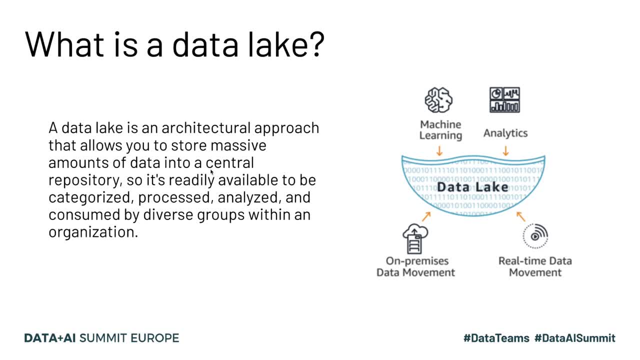 You can expect data to be accessed by machine learning, by different types of analytics. You should expect data to be loaded into Data Lake using the real-time movement, or you can have data coming from on-premises. The key is: the data needs to be readily available to be categorized, processed, analyzed and 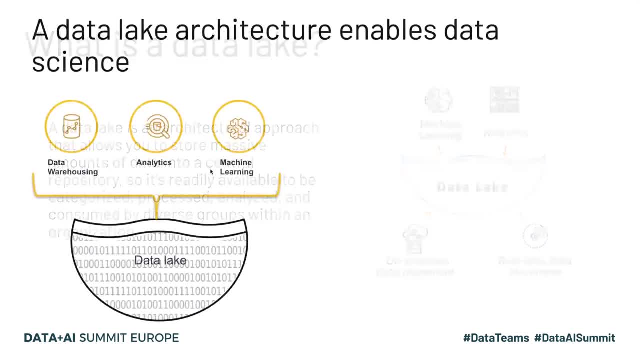 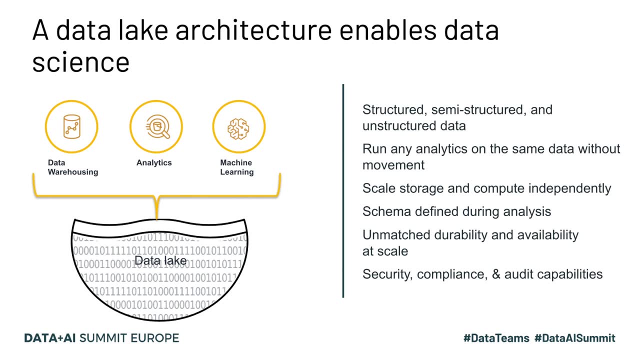 consumed by diverse groups within an organization. Today's Data Lake enables data science, but what can you expect from today's Data Lakes? You should expect structured and semi-structured, and structured data to be stored in the Data Lakes. You should be able to run analytics on the same data without movement. 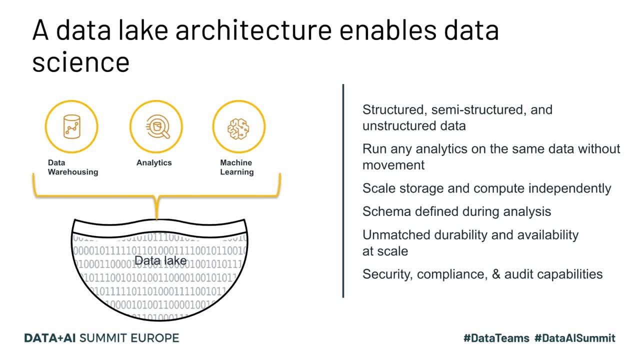 This is important in order to be able to scale your analytics. You cannot expect to move around petabytes of data. it puts stress on your network, potentially disrupts neighboring applications. You should expect your Data Lakes to scale, storage and compute independently. This is important for asymmetrical situations where you have a long tail of retention data. 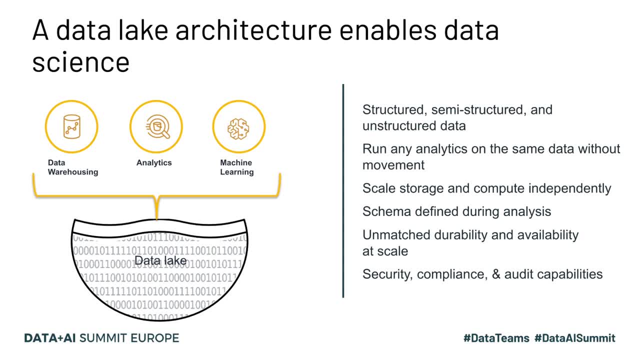 but, for example, using actively only a recent subset of data for machine learning. but you want to, for historical purposes, keep a longer-term data Understood trail. a longer tail of data Schema is frequently now defined during analysis. It's so-called schema on read. 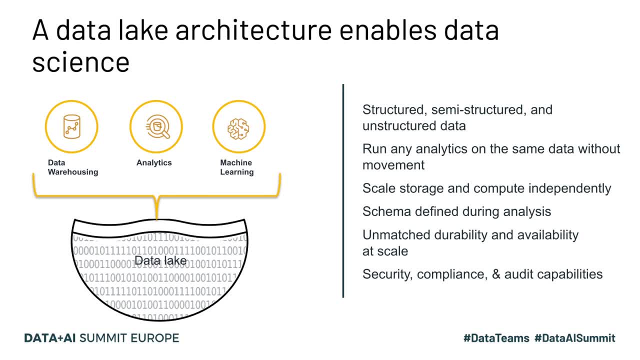 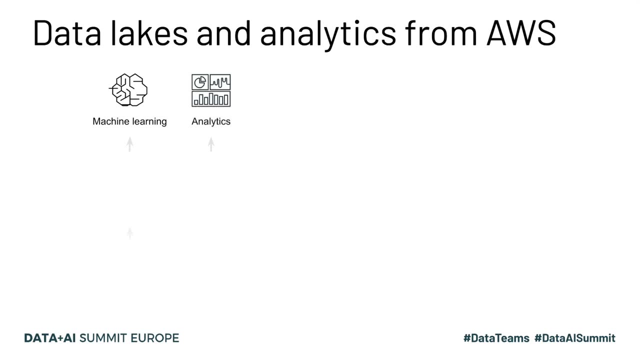 There is also expectation of unmatched durability and availability at scale, and you should expect also security, compliance and audit capabilities from your data lake, Data lakes and analytics on AWS. AWS offers open and comprehensive solutions. You should expect your analytics on data lakes and analytics on AWS to be secure. 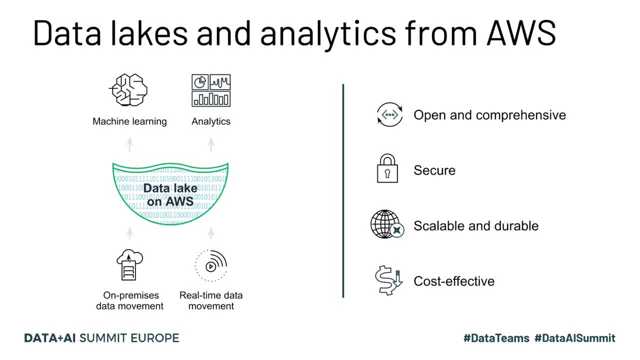 Scalable and cost-effective. You should expect to be able to load data from on-premises environment or you can expect movement of data, real-time data from streaming sources. You should expect data to be used in the data lake on AWS to be used for machine learning. 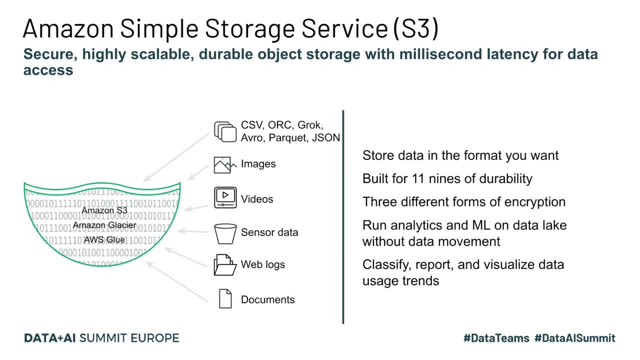 and analytics. There's one service I would like to highlight in particular that enables all of the analytics on AWS. That underpins all of the infrastructure of data lakes on AWS. It's Amazon Simple Storage Service. It's a secure, highly scalable and durable object storage with millisecond latency for 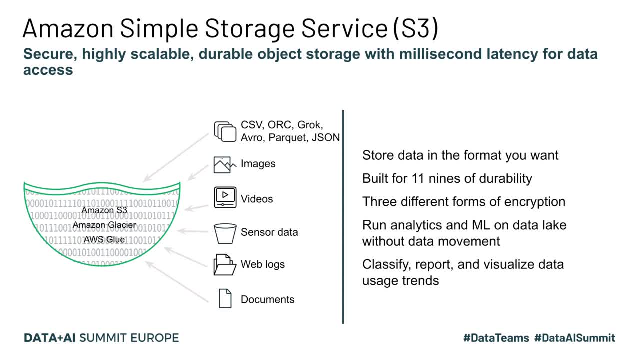 data access. You can store data in multiple formats, such as CSV, org, Avro, Parquet, JSON. It's built for 11 nines of durability. It supports several different forms of encryptions. You can run analytics or machine learning workloads on data lake without any data movement. 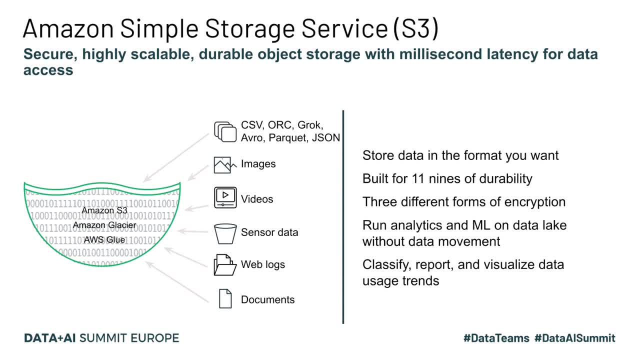 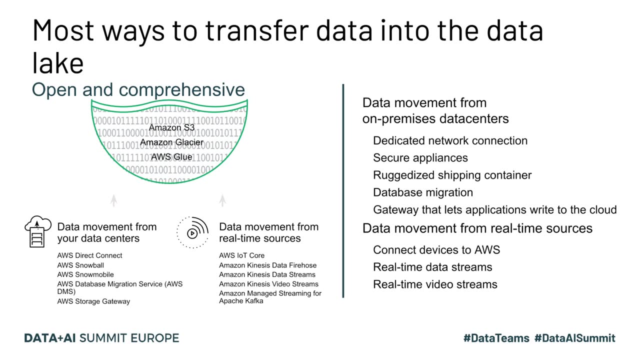 You can classify, report and visualize data usage trends. Variety of data includes images, videos, sensor data, web logs or documents. AWS offers the most ways to transfer your data into the data lake From on-premises. you have ability to establish dedicated network connections using services. 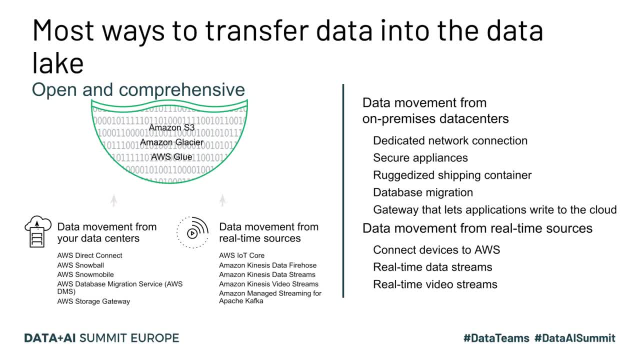 such as AWS Direct Connect. They're also secure offline. You can use them to transfer your data, such as AWS Snowmobile and AWS Snowball. There's also Snowball Edge. These are ruggedized shipping containers that you attach to your network. load the data. 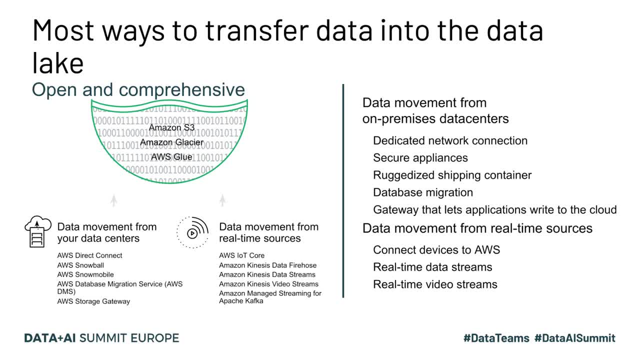 and ship them to Amazon data centers. that will load the data onto S3. There's also database migration service And a gateway. It's an AWS storage gateway that lets your application write directly to the cloud Data modes can be done also in real-time. 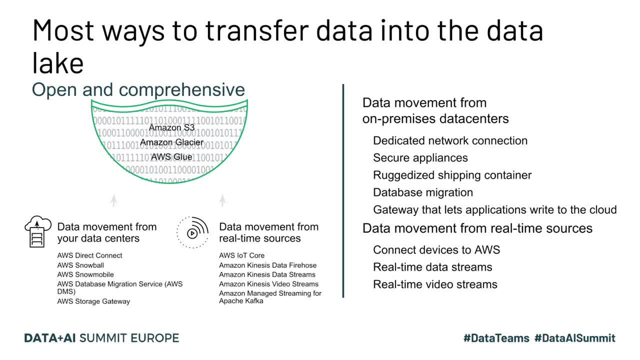 You connect devices to AWS using IoT Core. You can push data via through the real-time data streams or video streams with Kinesis Data Firehose or Kinesis Video Streams. If you are using Kafka, you can take advantage of Amazon Managed Streaming for Apache Kafka. 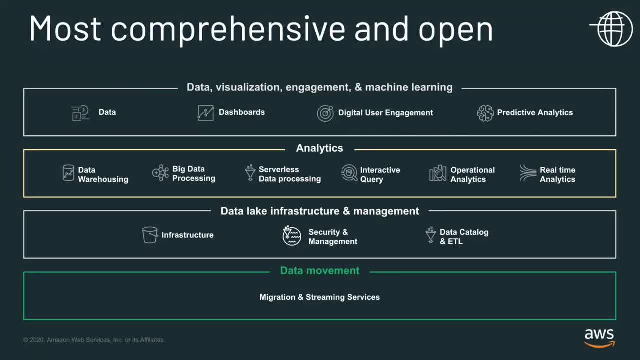 Amazon offers you the most comprehensive and open portfolio of machine learning and data analytics services. You can think about this portfolio as these four different layers. At the top you have data visualizations, dashboard, digital user engagement services, predictive analytics. So for predictive analytics, you can use SageMaker for dashboards, for example. 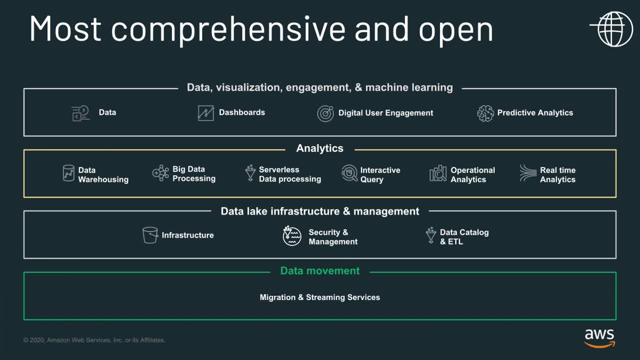 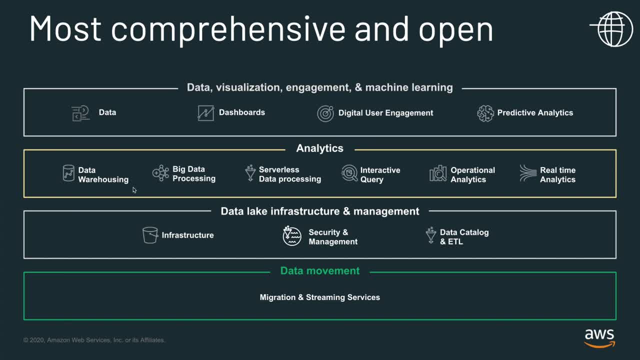 Analytics. You can use services such as Redshift for data warehousing. You can use serverless data processing with Lambda, interactive queries with Athena, operation analytics with Elasticsearch, real time analytics with Kinesis. There are also infrastructure and management and services associated with Kinect. 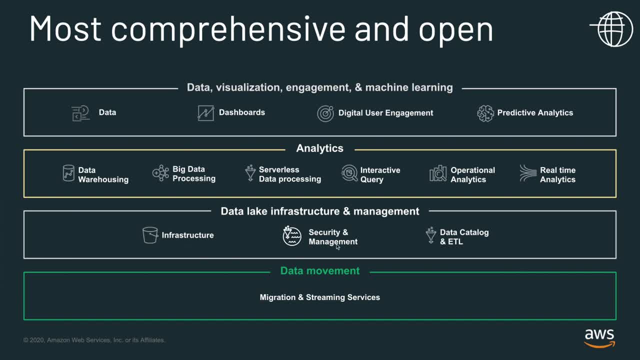 associated with that layer. you have your s3, you have a lake formation with security management and a glue catalog and etl and, of course, there's migration and streaming services and, if you think about this, these services and i i'd like to think about databricks as a this is cross-cutting. 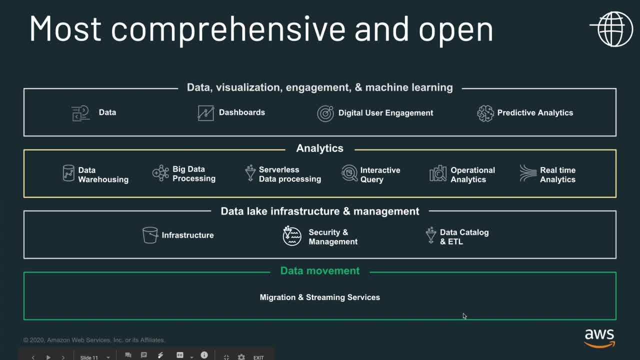 service that goes across all, all three layers, all four layers of the database, into data lake, do etl, do analytics and train machine learning and publish the and then produce data for your to power your dashboards. and with this i'd like to hand off back to brian. 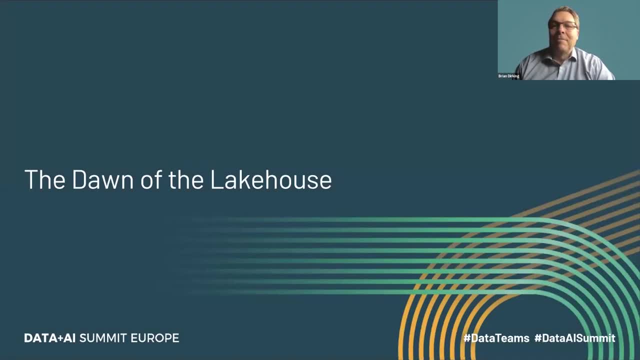 okay, thank you, igor, and now i will turn it over to dennis. hi, everyone, my name is dennis dubow and i'm the aws partner and solution architect manager covering the us at databricks. i'd like to thank igor for sharing the information and the work you're doing, and i'd like to thank you, igor, for. 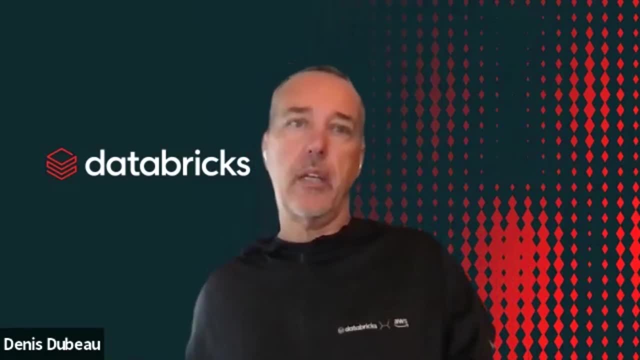 sharing your time and your time with us today- thank you, and we'll see you in the next session- is insights on the role of the cloud data lake. but now i'd like to switch gear a bit and describe this new lake house data management paradigm that many of you have heard lately. 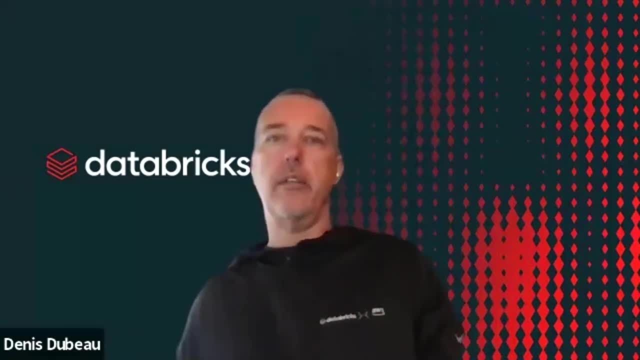 i first have to explain and touch upon on the history of the data warehouse industry. this is the background. so, since its inception in the late 1980s, data warehouse technologies have continued to evolve in these these large mpp mass, you know, massively parallel system architecture have led us where they can handle large amounts of data sizes really dedicated to 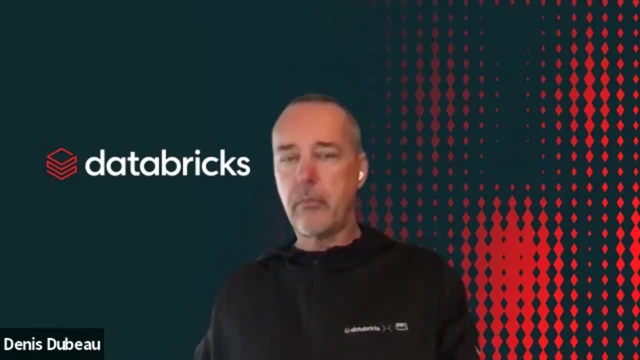 decision support and business intelligence application. now, while the warehouses were great for structured data, a lot of modern enterprises have to deal with unstructured data, semi-structured data and data with high variety, velocity and volume as well. data warehouse are not really well suited for these, for these use cases, and they are certainly. 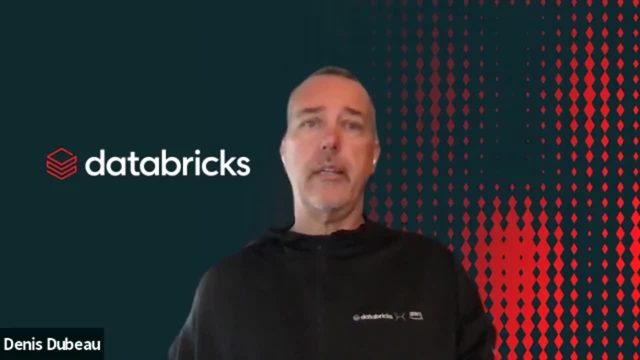 not the most cost efficient. then, about a decade ago, a company began building data lakes- large repositories of raw data in a variety of formats. many companies have invested in hadoop systems as well, as you might know. while data lakes are very suitable for storing a large amount of data in a cost-effective manner, 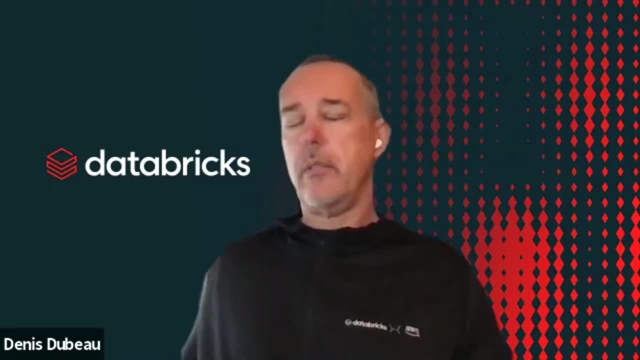 they lack some of the critical features, like the support of transaction boundaries, for instance. they do not inherently enforce data quality, and the absence of transaction consistency and isolation makes it almost impossible to mix a pens and reads, batch and batch and streaming jobs. so what is la cows really well, i would summarize it as a new system design which is basically: 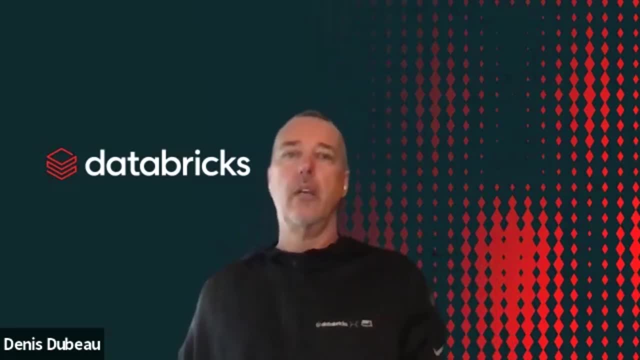 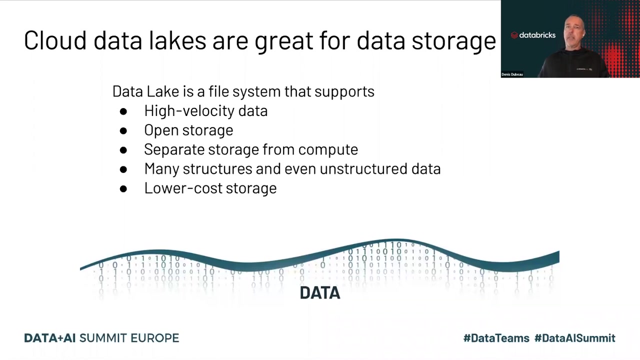 implementing the similar data structures and data management features uh to those in a data warehouse, while leveraging all the aspects and features of the data lake. Let's talk about the role of the cloud data lake. So really let's dive a little deeper and really look into the promises of the cloud data lake. 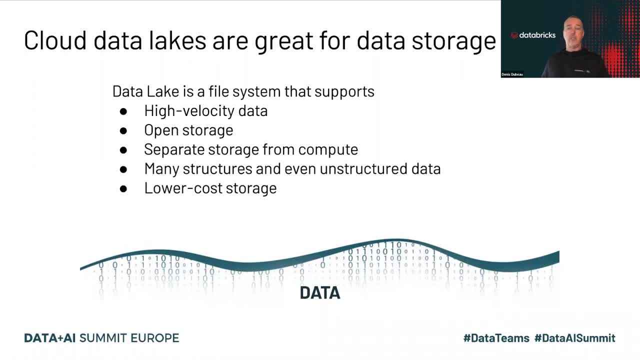 So cloud data lakes are great for storage, since the file system can store a wide variety of data types, as we just discussed, The data could be in format: transactional image, video, speech, web logs, IoT data, any other types of streaming data that can quickly be ingested and stored. 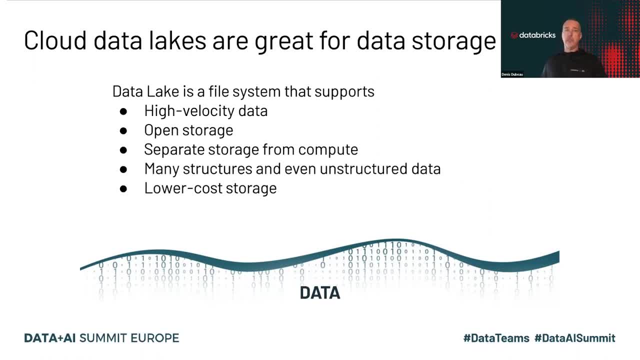 They provide an old storage format, which means that they can choose and take advantage of the most commonly adopted file formats like Parquet, JSON, CSV text, and access that data via multiple applications or services. You're also able to separate your storage. 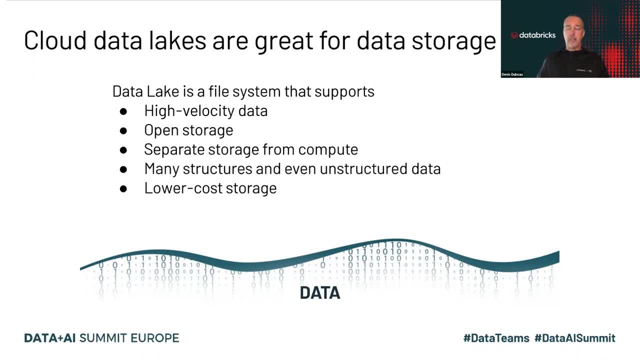 from your compute so that you can store all of your data in a single location and only provision the necessary compute as needed to process. So I mean I can't just really stress enough to store once in a single repository for all applications and just enough, just in time, compute resources needed. 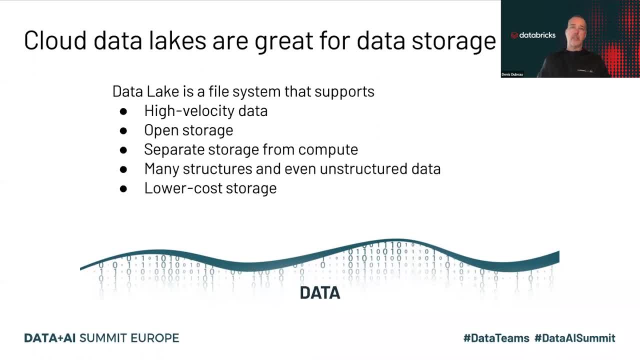 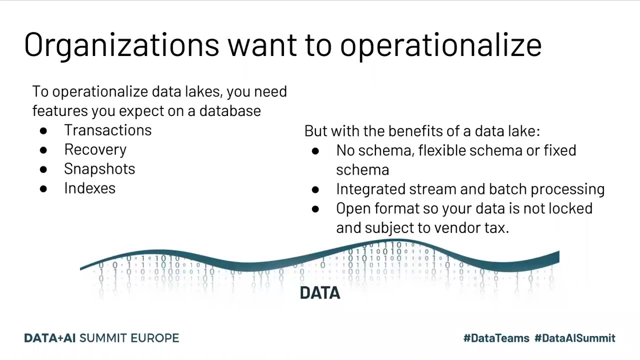 It also allows you to store many different types of structured and unstructured data sets I've referred to, and at the lowest options available as well. All right, So, and of course, many organizations want to operate, operationalize this data, So to do so, they often time need sophisticated features that you would usually expect from a relational database management system. 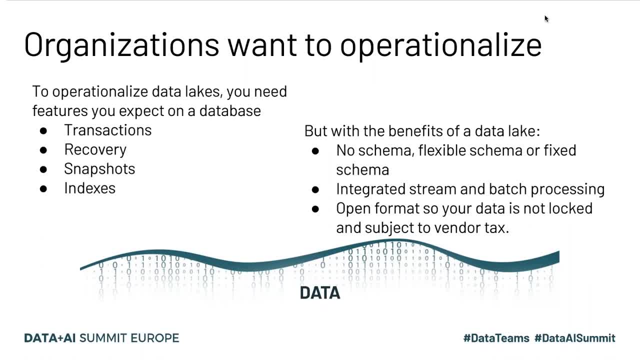 You'll want features like asset transaction, for instance, so that you can either, you know, fail or succeed at the transaction level. Ability, point in time snapshots and also create an optimized indexes is for very fast query access, While having all this benefit of a data lake, like having the flexibility of a scheme on read or even enforce a scheme on writes. and combine, simplify and unify the reliable. 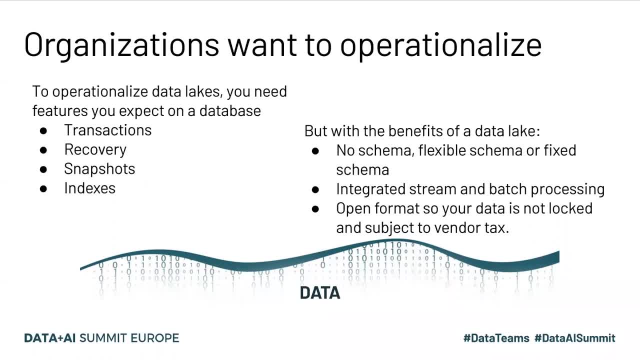 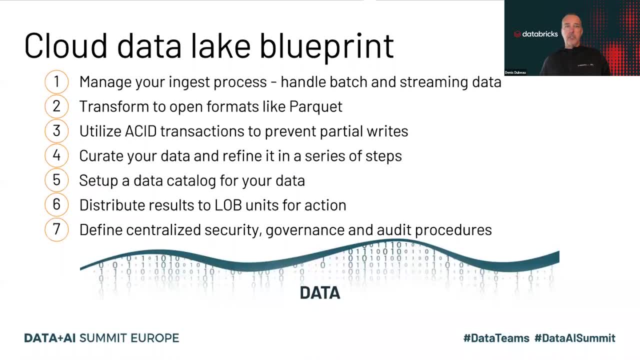 capability of streaming and batch processing, while keeping all of this in an open format With November login. So let's let's talk about the data lake cloud daily, And we found that there's our seven best practices that are universally well aligned with AWS, and this topic will cover it extensively. at reinvent last year, 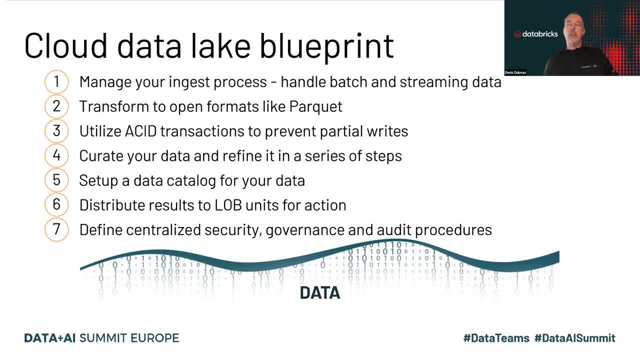 There is going to be many of those topics as well. they're going to be covered this year at reinvent as well. So you know, stay tuned on all the, the and the new features coming out in the database. But first let's go through these set of topics here. 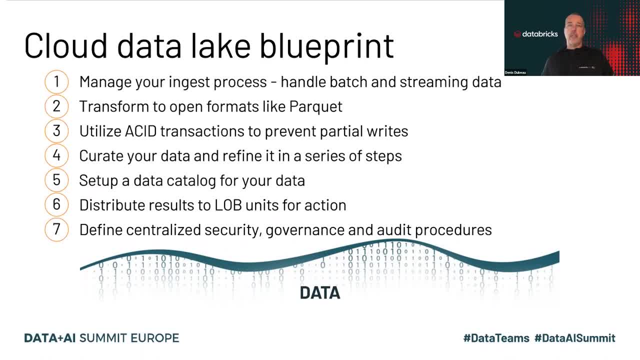 So, first, you wanna be able to reliably process streaming and batch data, as we've just mentioned, right? The second blueprint is you wanna make sure that you can transform to your data using an open data format such as Parquet, which is a platform and dependent machine readable. 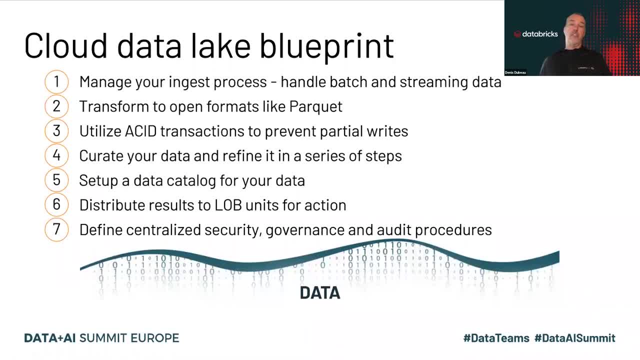 and specification that's published to the community Very open, no lock-in. Number three is to really prevent partial rights, basically having the ability to either roll back on failures to ensure integrity of your data And so that you end up having partially written data sets. 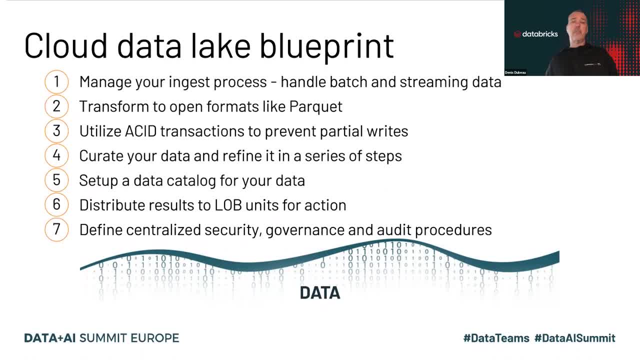 laying around in your data lake. Number four: you wanna curate your data and refine it in a series of step, following with a standard approach. really come in well adopted of framework in the industry. You also wanna be able to use an enterprise data catalog. 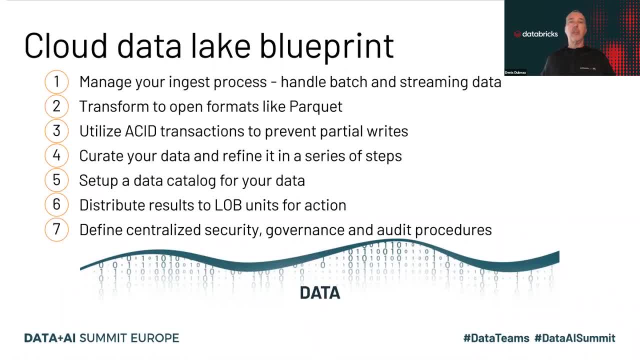 where you can catalog all of your assets and really in a centralized, scalable and secure repository that all of your services and tools can also access this metadata. So number six is really as well: run your business with the most secure cloud computing environment. 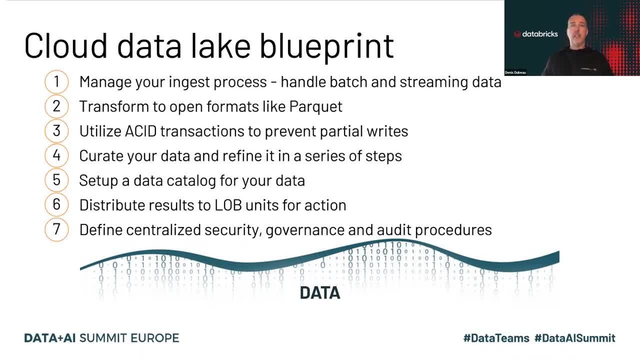 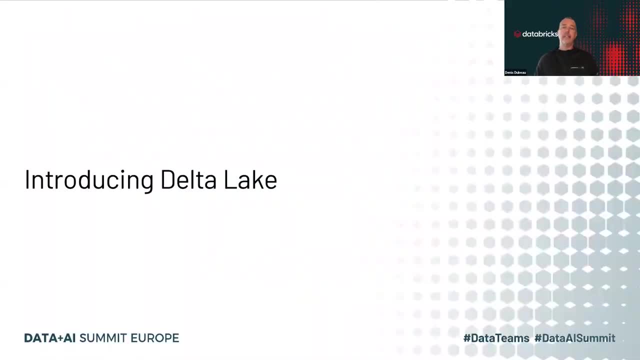 with the proper governance and audit procedures. Finally, you'll want to be able to distribute and publish your results to your downstream system and business applications to ensure that the proper actions are followed upon. So let's introduce the Delta Lake First. we're really proud to share the Delta Lake. 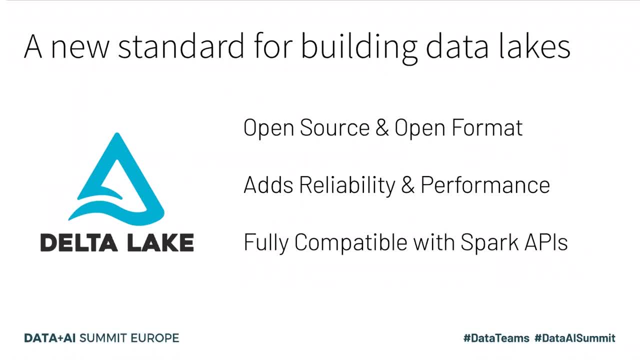 as an open source project hosted by the Linux Foundation, and that's also available if you follow deltaio, So all of the details are available publicly as well. Delta basically uses, as we've mentioned, an open source file format like Parquet. 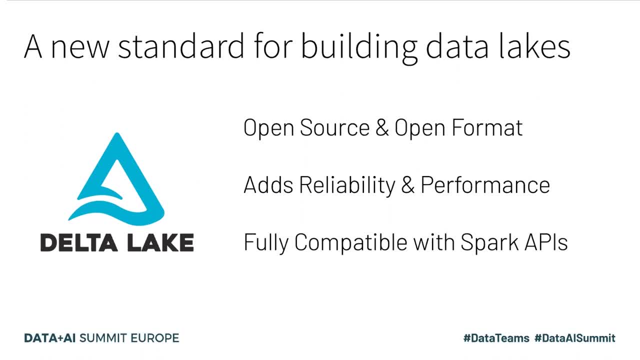 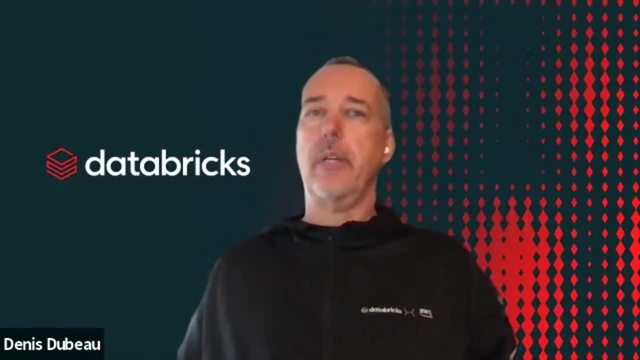 And we also provide a transaction launch which allows us to provide the reliability and the performance of a data lake while being compatible with Apache. So we're really proud to share this with you. So let's take just a few minutes here just to really cover. 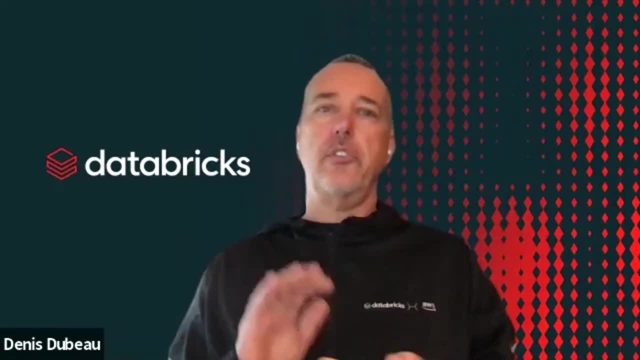 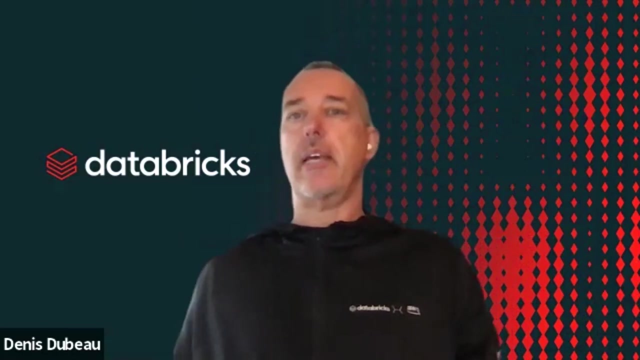 what I just said here is really is: there are two main parts to Delta. First, we version the Parquet files on your S3 bucket so that we can actually perform all the modifications on your data And secondly, we keep that transaction log. 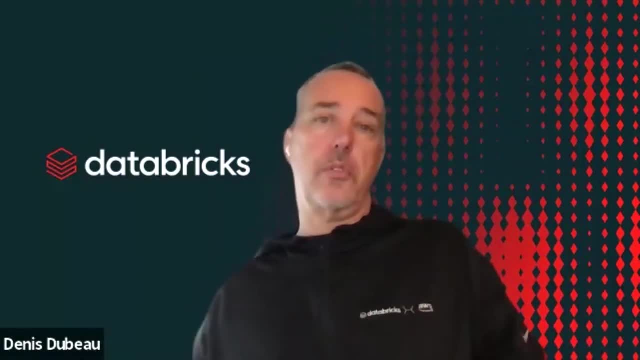 of all these operations, which allows us to also store those transaction log on your S3 bucket. So it's all leveraging S3, as well as leveraging Parquet, as well as having that transaction log. that provides us the reliability that you would expect from your data lake. 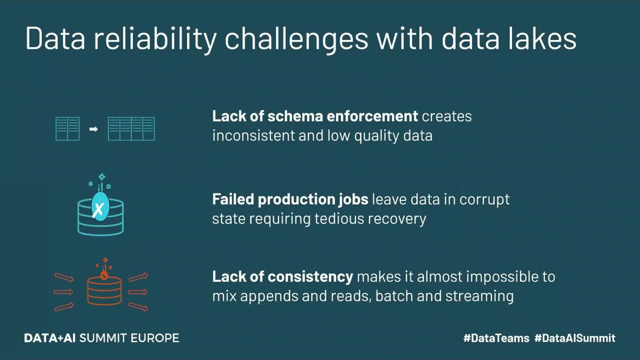 So let's go. and then you know why: Delta basically. So we found a numbers of different challenges with data lake Number one, Amazon S3, is a highly available, scalable and durable object store, but it's not, you know. 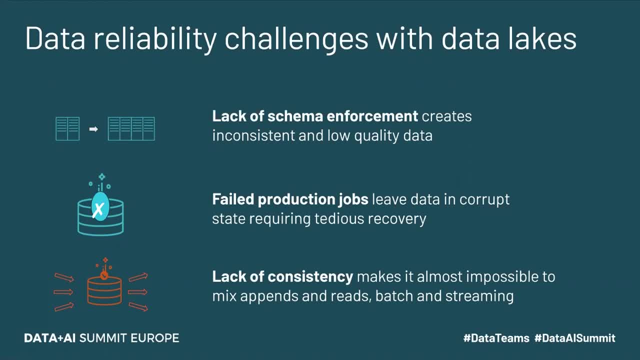 but it does not support object locking. So basically, as you are writing file content to a specific location, obviously that you have permission to, you can't really not enforce the numbers of columns or the data attributes when you're writing into an S3 bucket. 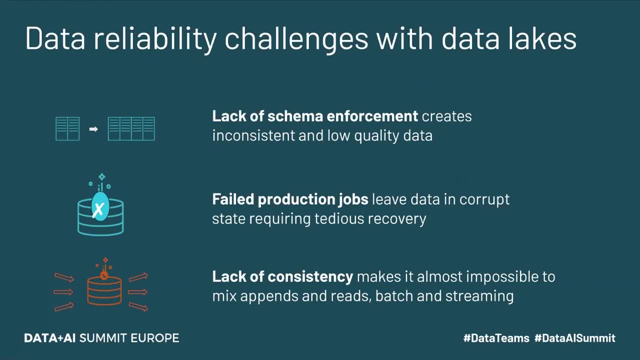 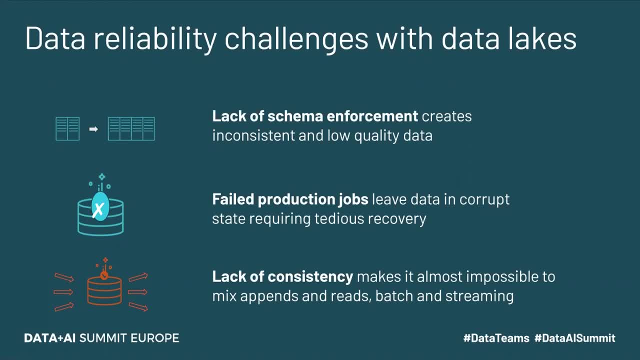 as you are running through. you know the set of these challenges. now you have been in an unreliable state where you might have possibly written partially content. you know partial content by. you know that are caused by those failures. Now you know you have to go through the manual process. 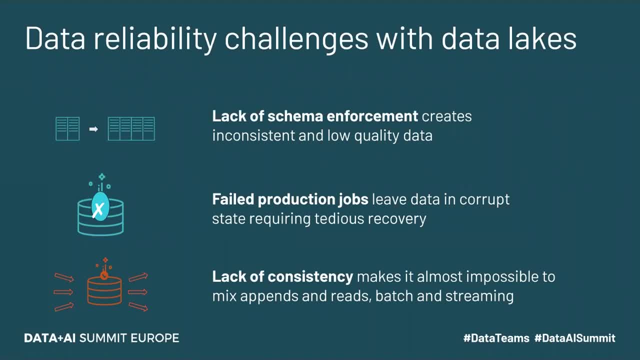 to run, that you know that data that's written and then rerun these jobs or these pipelines. And last, the last challenge here is also there is no awareness of transaction boundaries similar to what you'll find in an RDBMS. 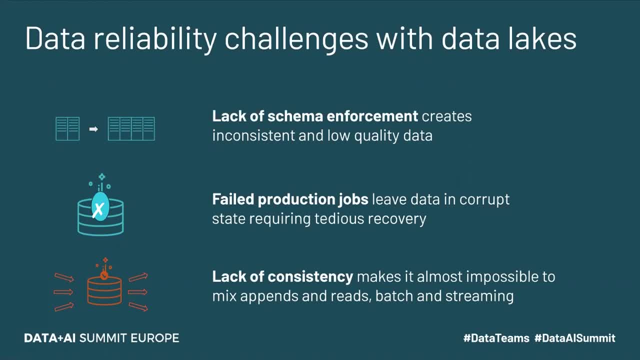 So there's no. there's no consistency enforced by the file system natively. So, consequently, it's very difficult and almost impossible to mix readers and writers to ensure consistency at an object level without building some very complex pipeline. And you know, and also you know. 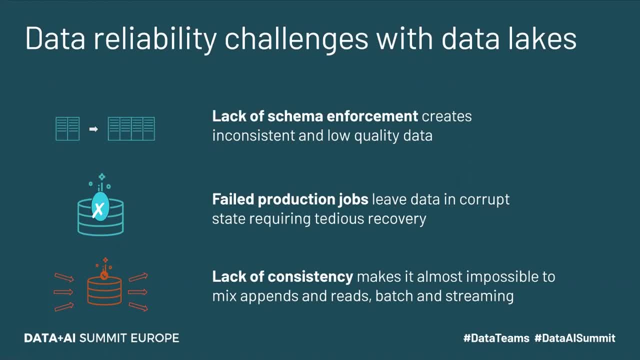 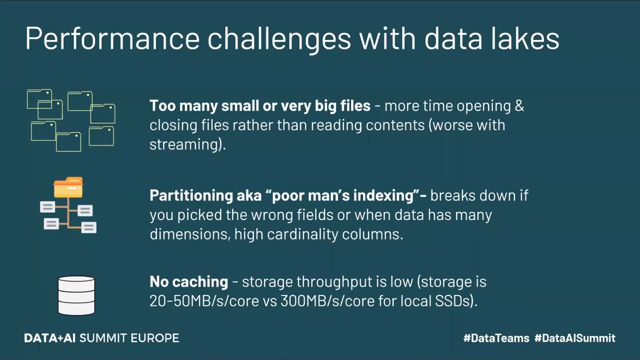 investing a fair amount of resources to do so. So that's on the reliability front, On the performance characteristics of Data Lake. you know you'll encounter, you know those two many small into. you know very small, very big files. 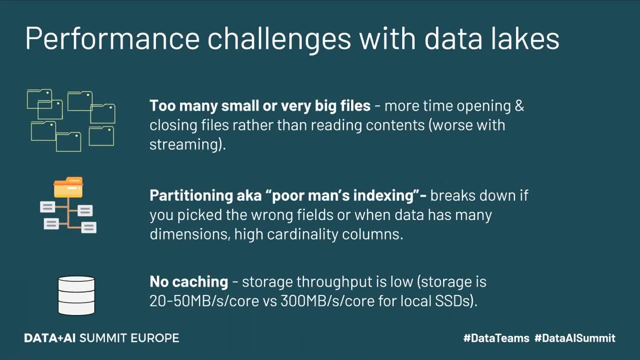 When you start streaming data, you're gonna have a large amount of very small files which you know, basically, is gonna really affect your performance. The partitioning strategy is really a poor man's indexing, as you will know. So once you decide the partitioning, 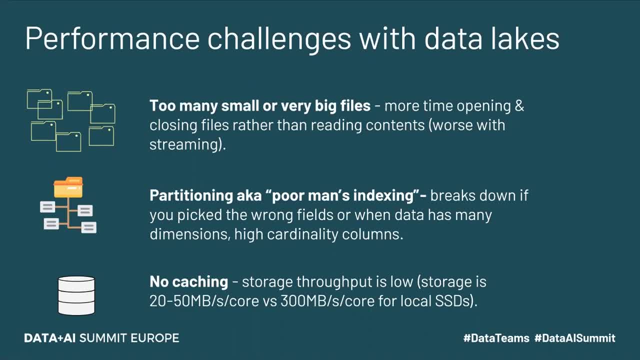 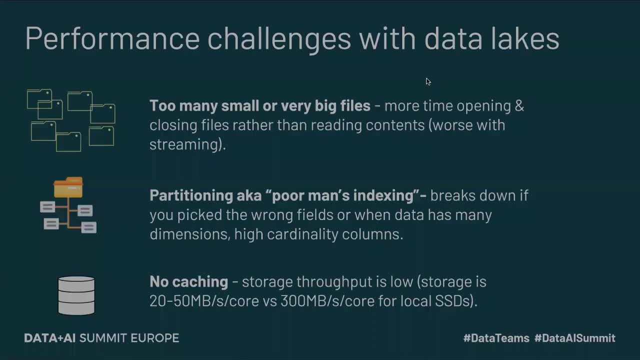 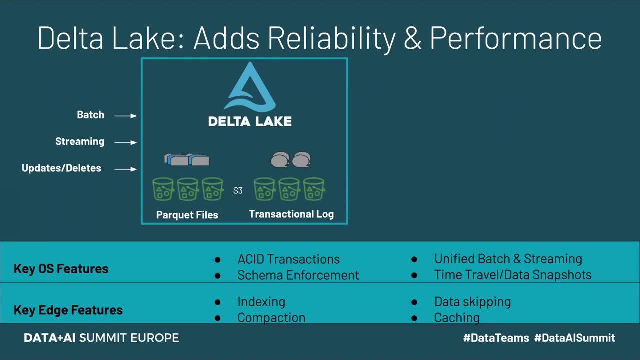 there's no really ways to build very strong and efficient indexes And there's really no caching available as well on the file storage. So let's talk about how do we ensure reliability using Delta Lake. So you know, I touched a little bit upon that. 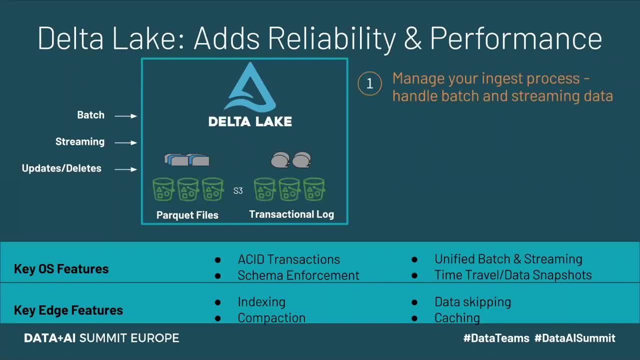 So we do offer a numbers of features, and one of them is the transaction log that we have. that's you know again that is written to your S3 environment and that transaction log sits on top of the Parquet file. 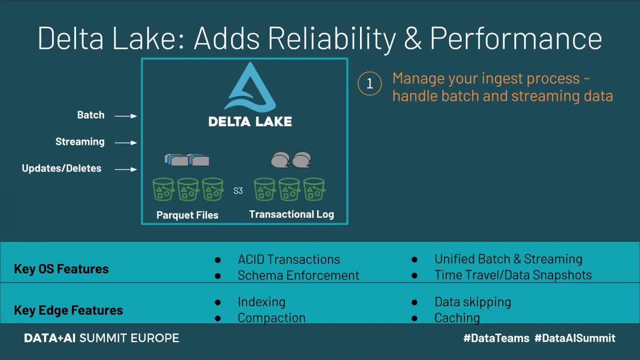 And really that's what Delta Lake's all about. right. So that transaction log allows us to really manage that batch and streaming data because we have the control over the transactions coming through. So there's a set of open source features that we provide. 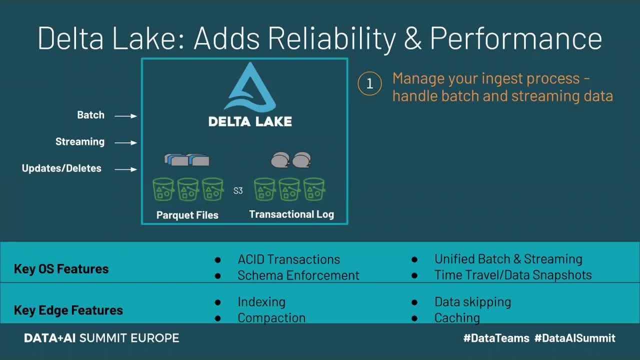 with the open source Delta Lake, And those features are the support of asset transactions, schema enforcement that we just talked about, ability to unify, batch and streaming, as well as time travel and data snapshots, because, you know, it's not just a matter of time travel and data snapshots. it's a matter of time travel and data snapshots, because you know it's not just a matter of time travel and data snapshots, because you know it's not just a matter of time travel and data snapshots, because you know. 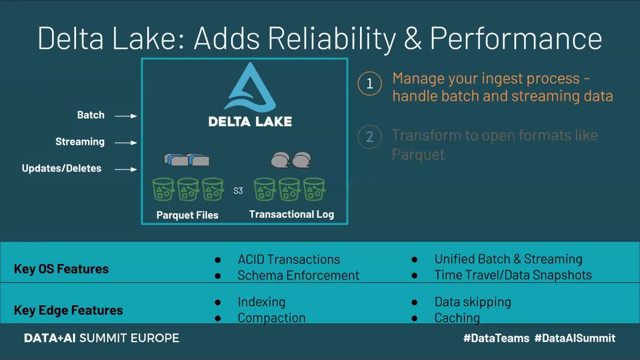 of the transaction log that we support. Now the. those are all open source capabilities. Now the. if you leverage Databricks and some of our, you know the commercial features of Databricks- you'll provide as well on top of these open source features. 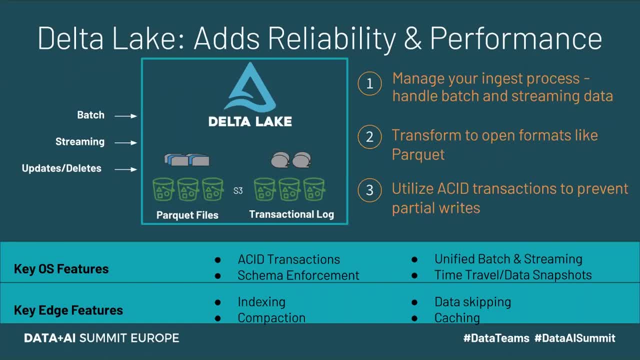 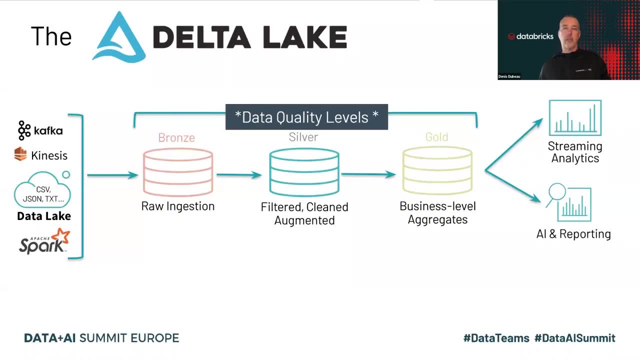 the ability to create very complex indexes, you know, and it will also provide auto-compaction, also the ability to do data skipping and caching as well. All right, So now that we understand the reliability and the performance features of Delta Lake, it's very simple and easy to implement. 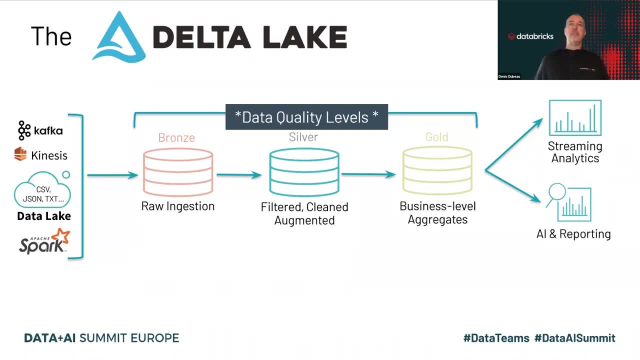 this commonly adopted industry framework where you ingest your data type from your raw sources and once we call this bronze layer, Now the bronze layers. I mean this is there's one image here, but you could have multiple bronze ingestion files. 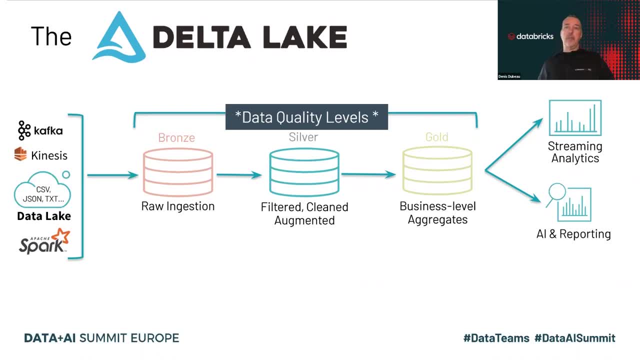 and then from there then you're applying your filtering and your cleansing criteria is to produce your silver layers And again, those are many, to many. So many bronze, could you know, feed into your silver layer and vice versa. And what we found is that most of our organization. 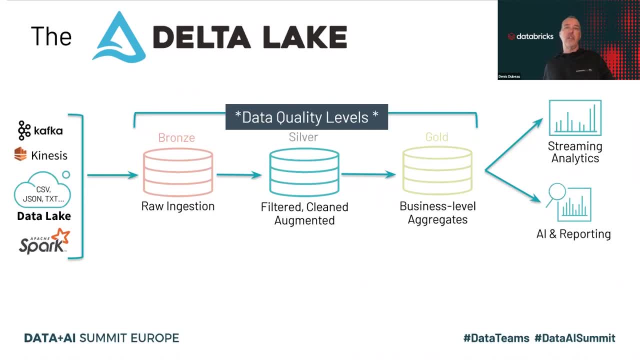 are then typically granting access to your silver layers so that you can start building those ML pipelines as well, providing you know all the data assets with a minimal. you know, you know the full curation process for to your, to your data scientist. 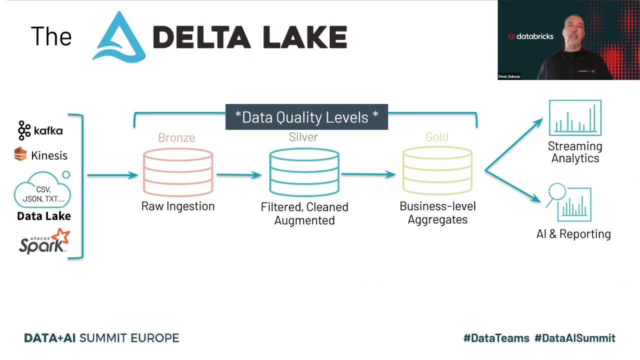 And then, as you move that data from silver to gold, then you really aggregate this data where it's become, you know, becomes what we call the serving layer of the data, which is that, that gold version where you'll send down to your streaming. 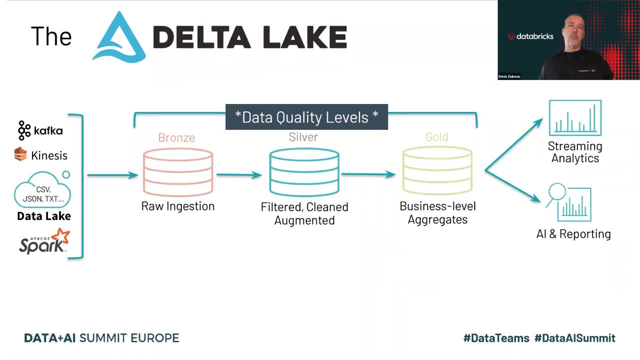 analytic systems and your, your reporting and NBI. So via the refinement process you'll incrementally improve the quality of your data until it's really really good for consumption by the serving end points and also allow the evaluation of the schema enforcement. 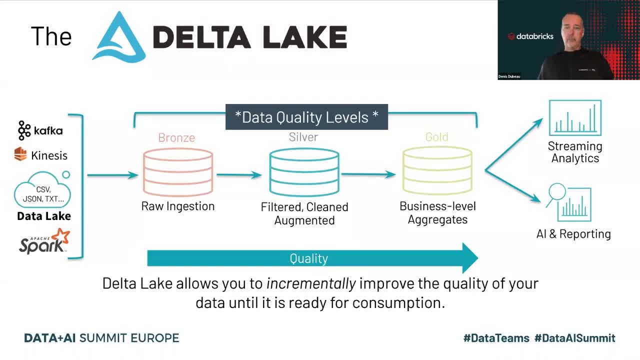 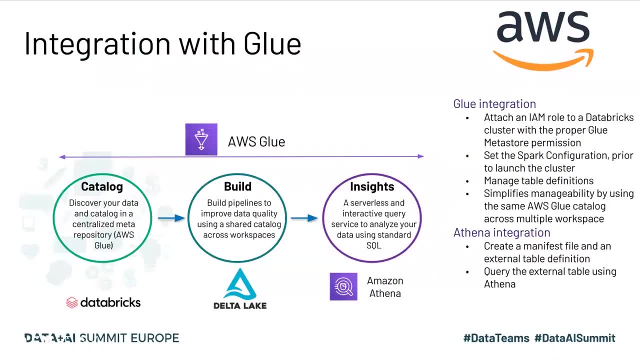 requirements throughout this layered framework. So the quality improves from left to right, essentially All right. So there's a numbers of integration point on the landscape and I want to touch on a few of them. One of them is glue, So let's talk about the Databricks level. 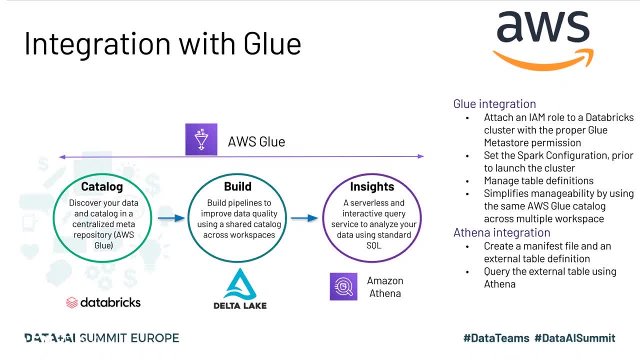 and integration with glue And you know, obviously as an enterprise, as an enterprise Metastore, it's really easy to leverage glue today with Delta So you build your pipelines, you can store all your metadata And so that you can discover that data quality. 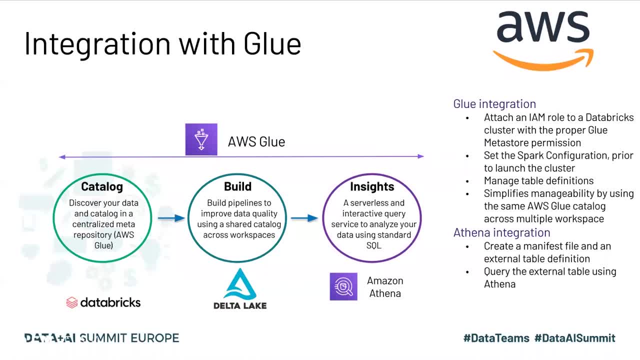 and the shared catalog assets as you're building these different pipelines Now. once you have this data catalog in the enterprise glue Metastore, it is really easy then to start consuming your data from- from Athena's point of view As well. 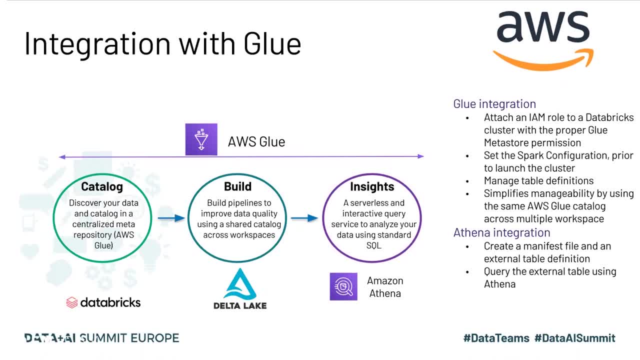 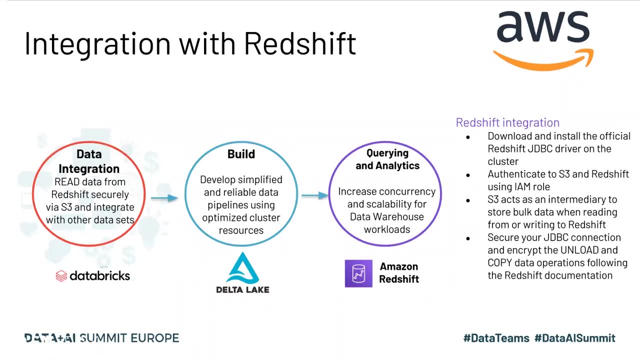 So it's full integration with glue and Athena via the Databricks unified data analytics platform. The next integration I'd like to talk about is the Redshift integration. So Redshift today supports the ability to query data, So Redshift spectrum allows you to read Delta Lake tables. 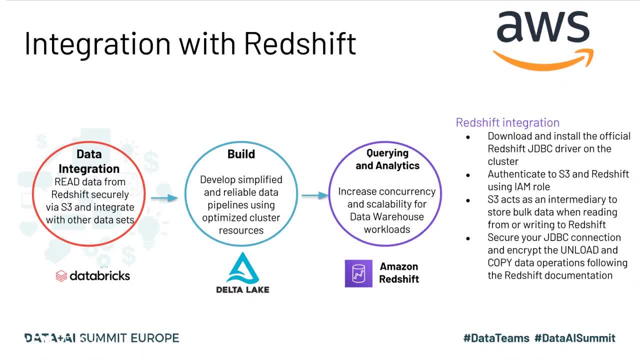 directly And we can also take. we can also take the data from S3 and then push that goal data set value directly into your Redshift instance, If you prefer to serve it this way, from a dashboard or from a, you know, data warehousing workload characteristics. 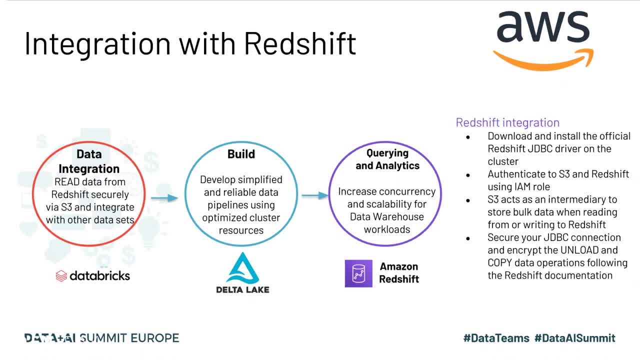 So it's really providing that ability to start serving data to your downstream custodian so that it can actually make the business decision of the curated data. So then again back to the blueprint. that's the number six item that we talked about, about distributing our results for line of business. 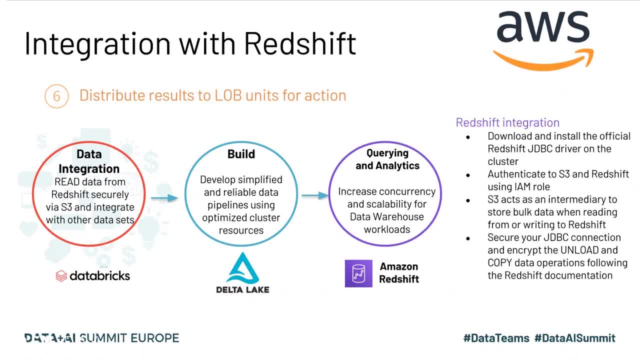 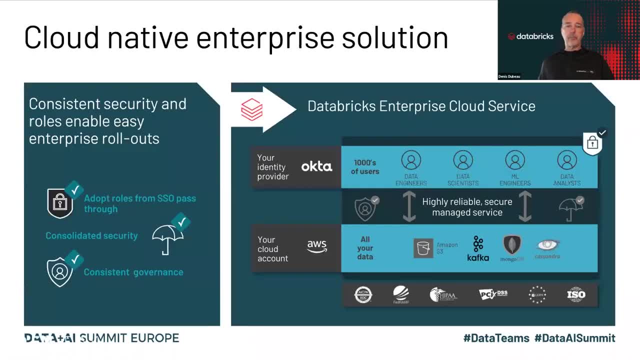 So, whether you're using Athena or Redshift or another RDS type, so layer, we have those two integrations. from a Databricks standpoint, the first part of the services on AWS- We also do this in a very cloud native enterprise solution. 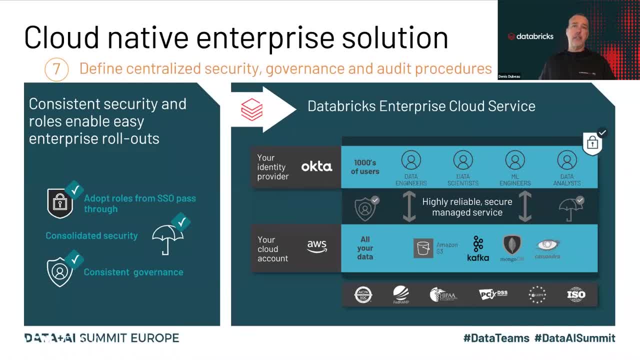 So we centralize all of our assets, leveraging all the identity access management and as well as all the AWS services to secure this content, whether it's the data and transit data at rest or as well as preventing, you know, access to these different environments and following all the 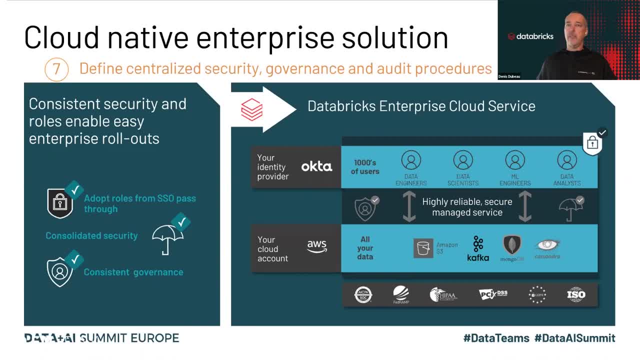 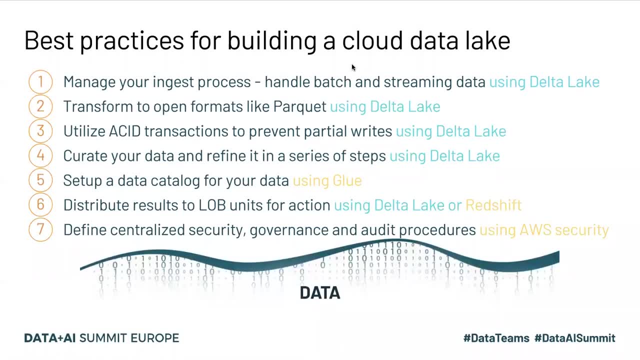 best practices and security and consistent governance and approaches. So, in a nutshell, if we review, if we review the what we've just talked about, we basically hit on all of those seven best practices. Now, reviewing those, I you know. 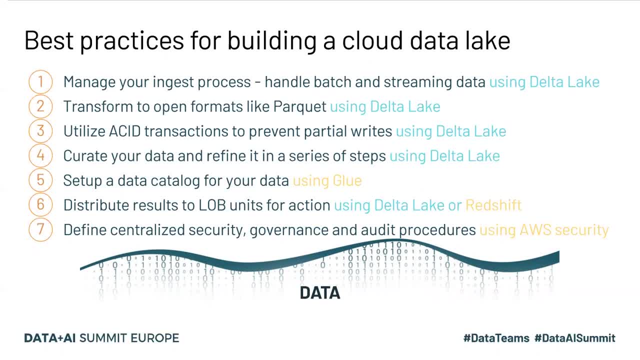 the, the, the seven items. all of these items are addressed either using Delta Lake on top of your data Lake on S3 and integrating your catalog at the enterprise leverage, leveraging glue and distributing your line of new data to your line of business. 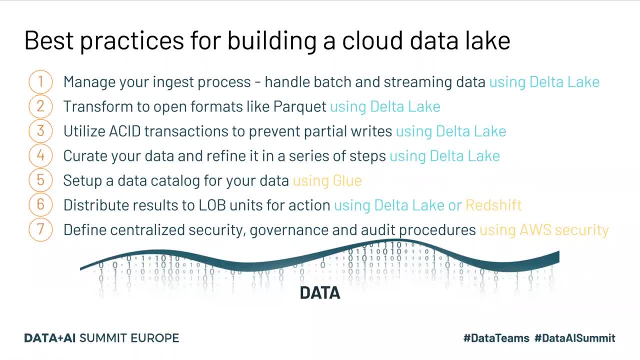 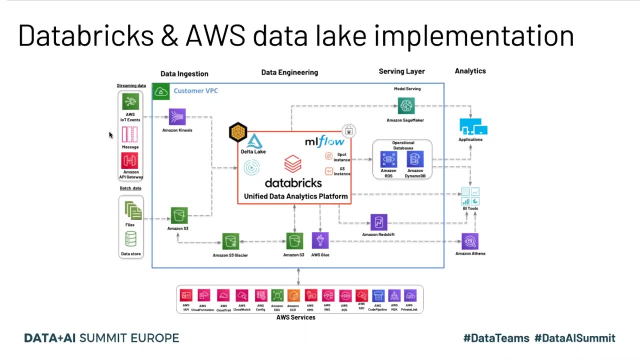 whether it's through Redshift, whether it's through Athena, and all of this done in a very secured and governed and an audit audited processes. So a very well integrated solution. So let me just kind of wrap this up here and provide you this overview of Databricks on the AWS landscape. 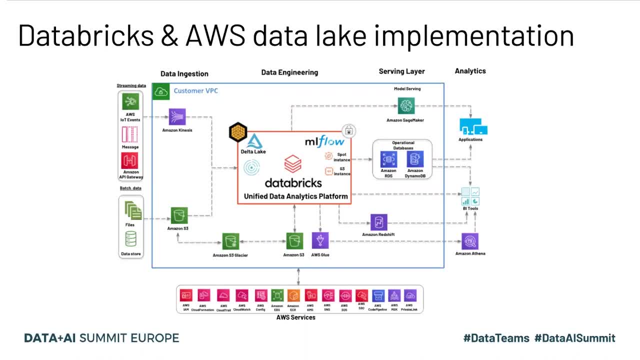 Now a couple of, if you look at those four pillars, either from ingesting data to the data engineering layer, to serving the data and for the addicts to be consumed. we integrate when a numbers of first-party services, whether you're looking at Kinesis for in, for steaming ingestion, or the 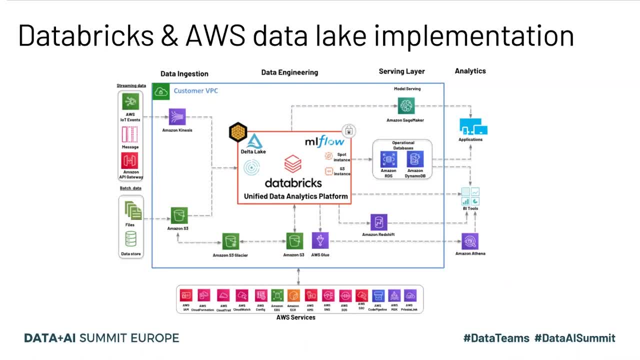 managed Kafka solution as well as obviously ingesting data directly from from S3, either this could all be done by, you know, other services, like Apple, for instance, or or third-party solutions as well. So this data can can now be ingested within the boundaries of the customer's VPC. 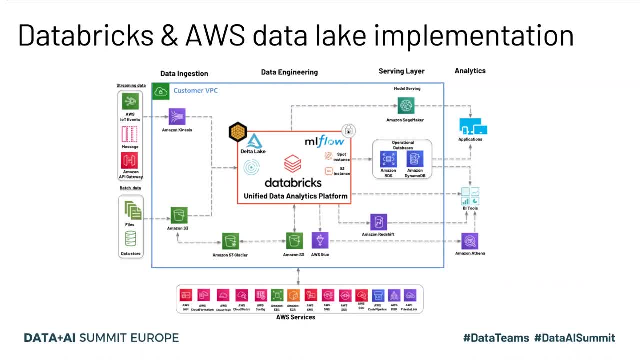 So all of these Databricks, cluster instances, are spun up in the clusters in the customer's VPC, interacting with your S3 data lake directly, and then Delta Lake sits on top of your S3 object storage And, as I said earlier, 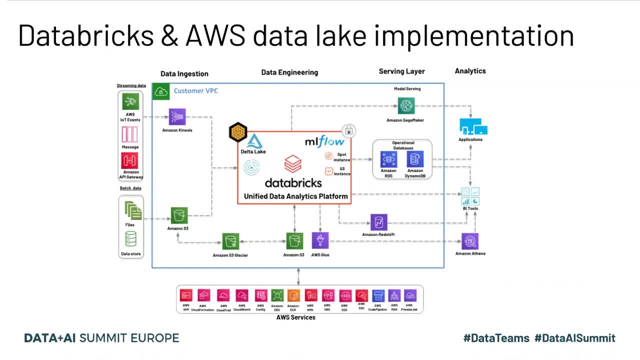 S3 parquet file with a transaction log that provides you that real reliability and performance that Delta provides you by interacting with your your, your local, your, your data locally. We also provide you a numbers of supportive spot instances and since types as well, that are available today on AWS and provide this best of breed of separation.